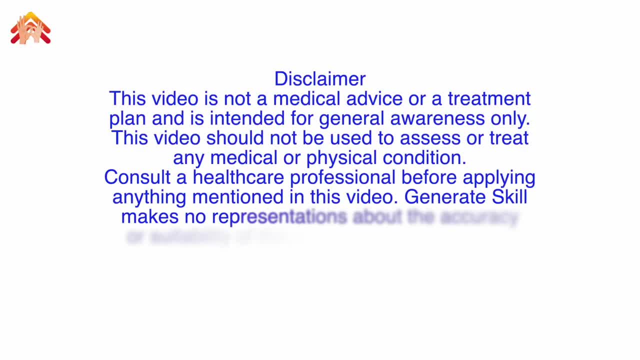 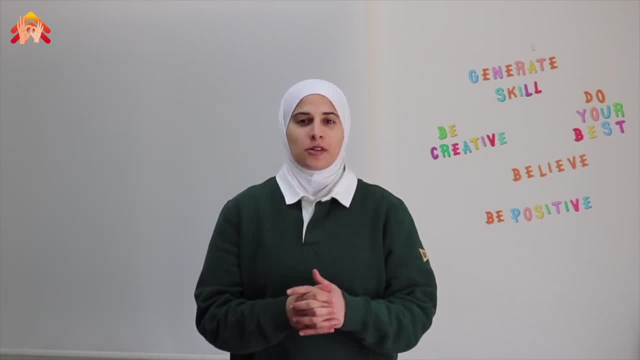 Balance is a huge topic and I can't talk about it for hours, Though I'm going to share with you some important information about balance skills and then I'm going to show you the best balance activities you can do with children. Hello, this is Tamara. I'm a pediatric physiotherapist. We, as physios, consider balance skills one of the most important motor milestones children acquire. We expect from children by the age of five years to acquire all the basic balance skills. Why having sufficient balance is so important with kids? Having good balance allows a child to walk independently on different types of surfaces. 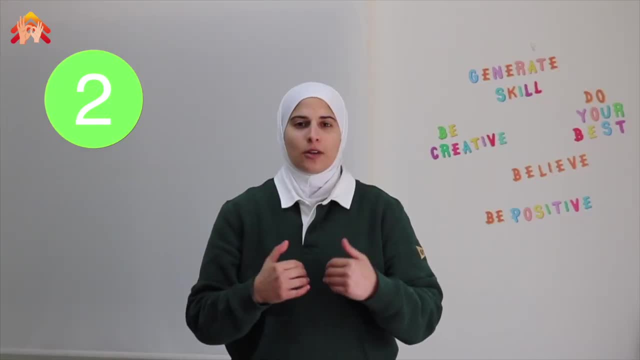 whether it's indoor or outdoor. Having good balance allows a child to maneuver independently in any environment with any physical demand, such as going up and down the stairs or walking on the curbs, or walking on the stairs Or using the sidewalk. 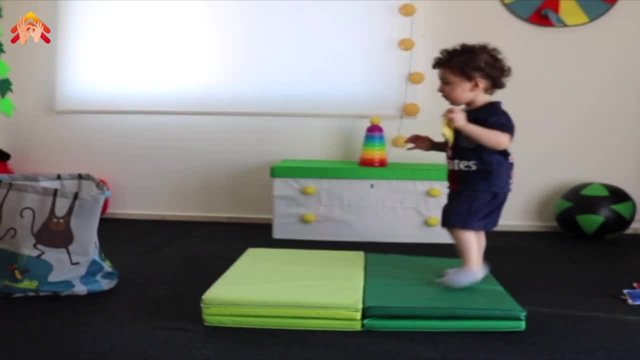 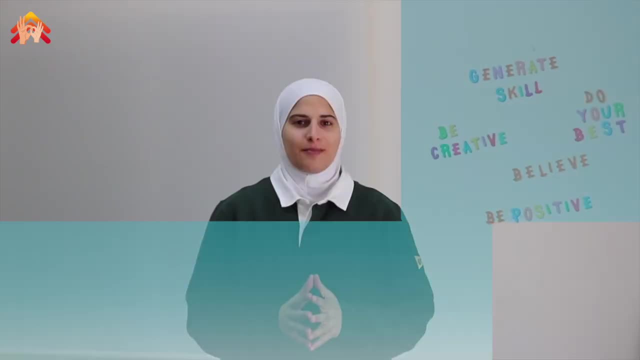 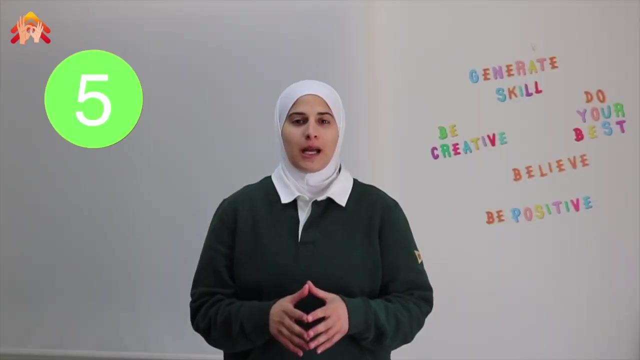 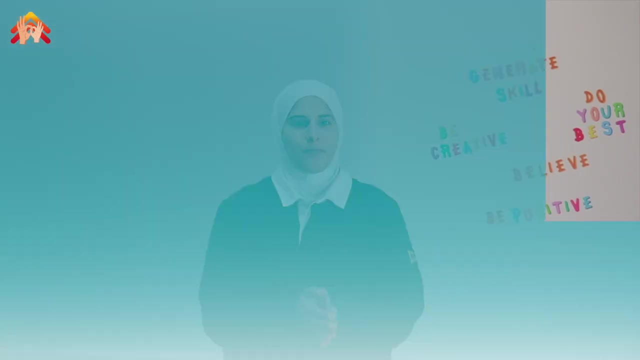 Also, children with proper balance are confident enough to play independently with their siblings and peers indoor and outdoor, such as swinging and sliding. Furthermore, having good balance should prevent children from frequent falls and injuries. Balance skills are the basis to acquire many gross motor skills, such as jumping, running and ball play. 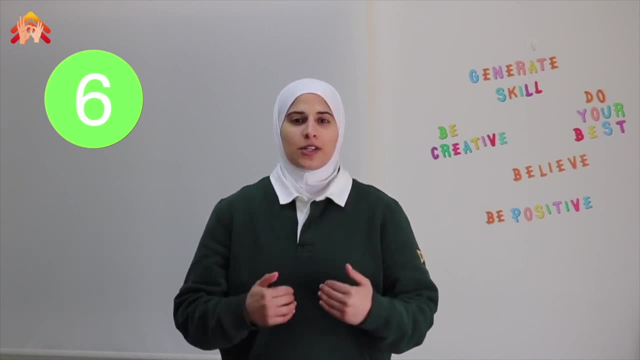 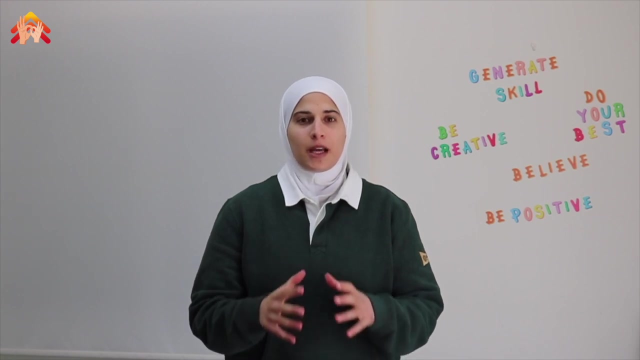 Having said this, and moving to the last point, having sufficient balance skills will allow children to learn any sports they prefer that require the whole body movement, like tennis, football, basketball or any type of martial arts. Any medical problem that causes developmental delay will ultimately cause delayed and imbalanced skills. 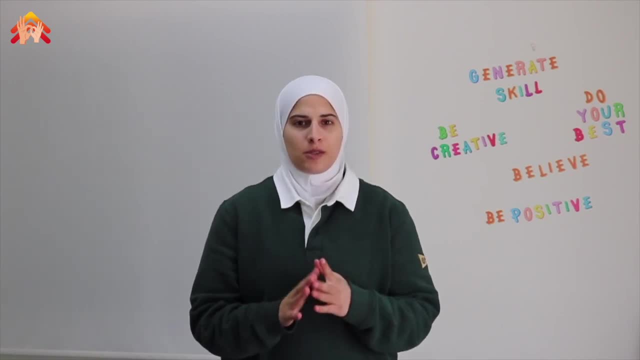 such as cerebral palsy, Down syndrome and autism spectrum disorder. Therefore, delayed and imbalanced skills is a common issue we see as pediatrics problems, So let's work all together and help children improve their balance. The question is how to improve children's balance. 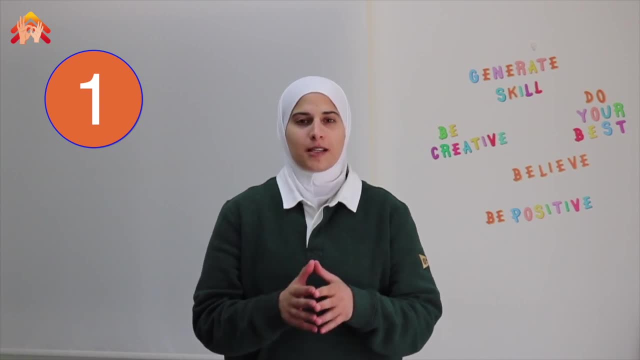 The first and most important thing is to assess and treat any medical issue that causes delayed and imbalanced and can be treated, such as vision problems and inner ear problems. The second thing is to strengthen weak muscles, especially the core muscles. You can find in the description below links to a number of strength exercises. 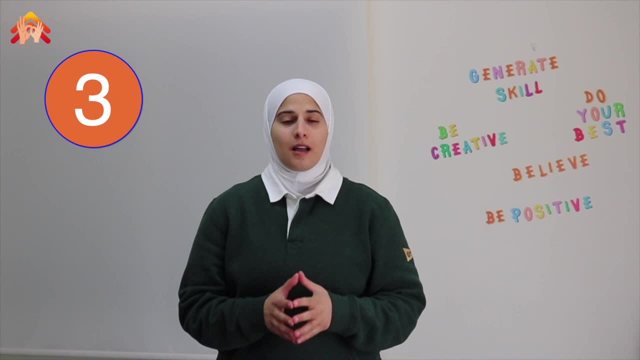 for children. The third thing is to practice on balance. The good news is I'm going to demonstrate 57 balance activities you can do with your kids at home or in any environment, using simple equipment. Don't worry, because if you don't have any of these equipment, 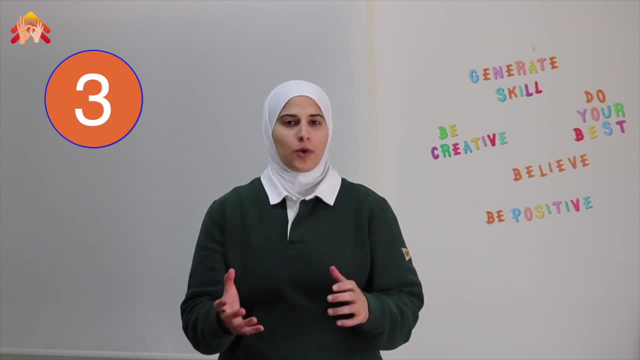 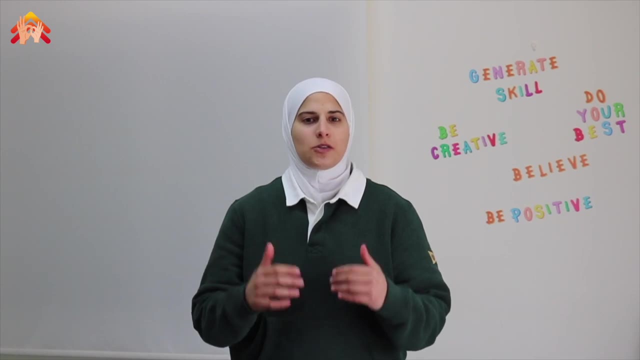 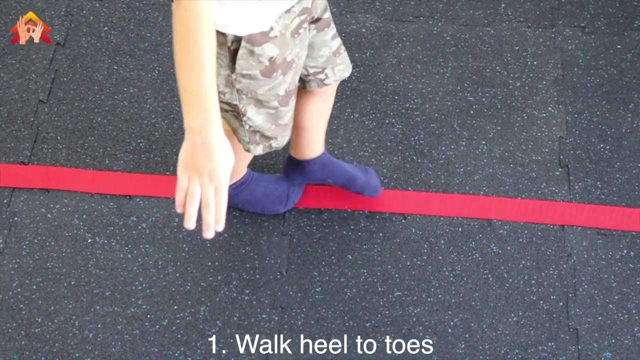 I'm going to show you many balance activities you can do with your kids without any equipment. Make sure to watch all the activities to have as many ideas as possible. You will see that I am playing with my right hand. They're my hands. 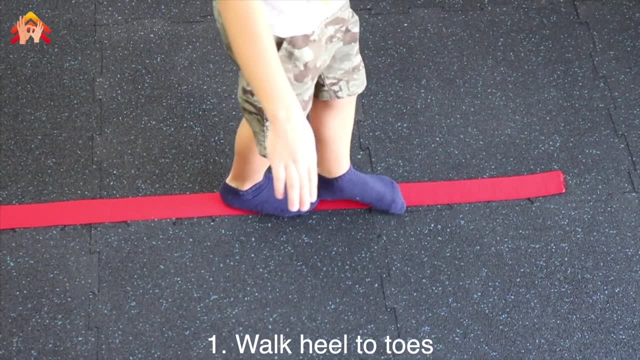 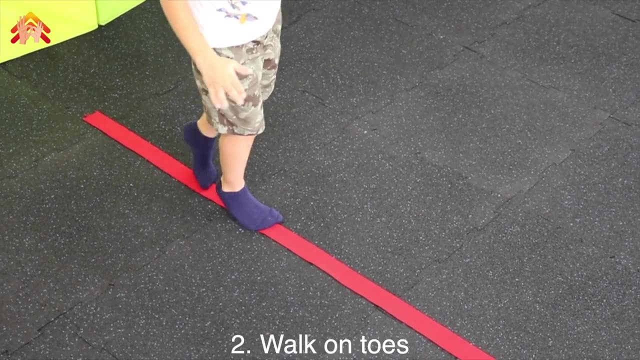 In this little space. my right hand is my body, My left hand is my back, The right hand is my shoulders, The left hand is my feet. This is my arm. The left arm is my side of my head. This is my foot. 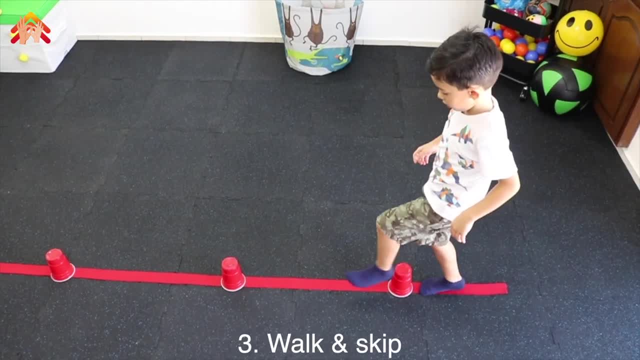 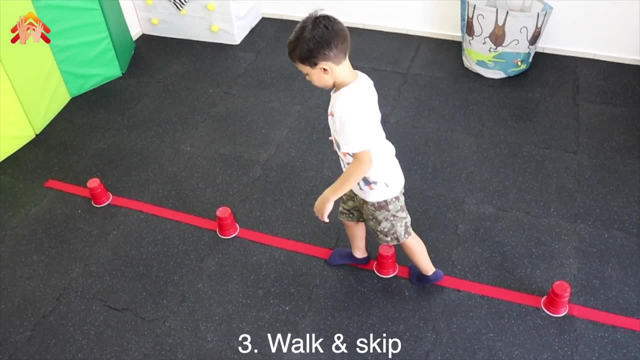 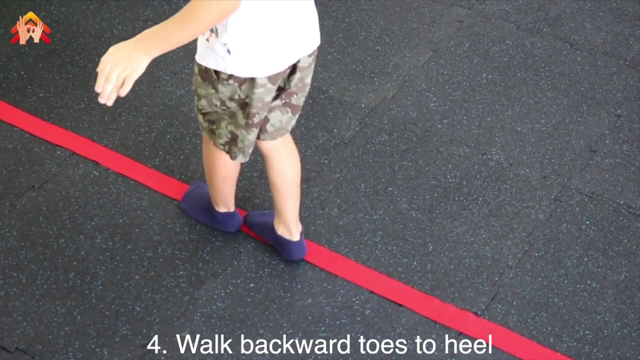 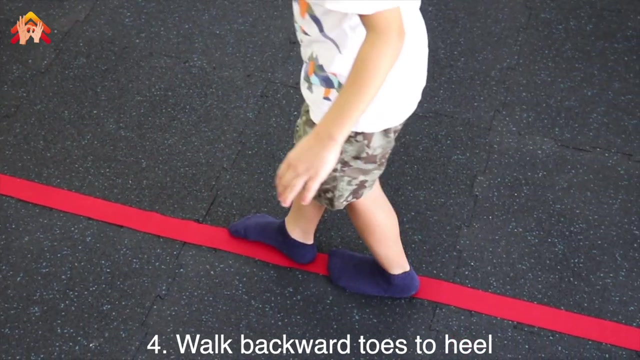 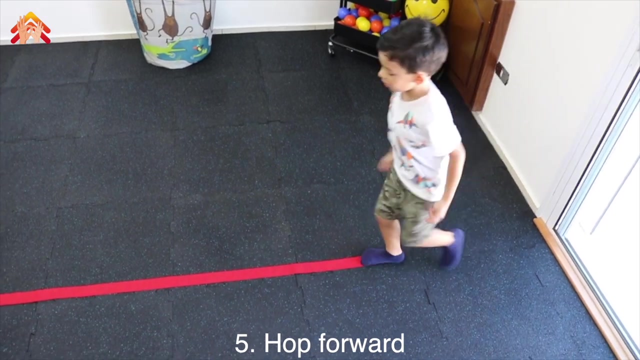 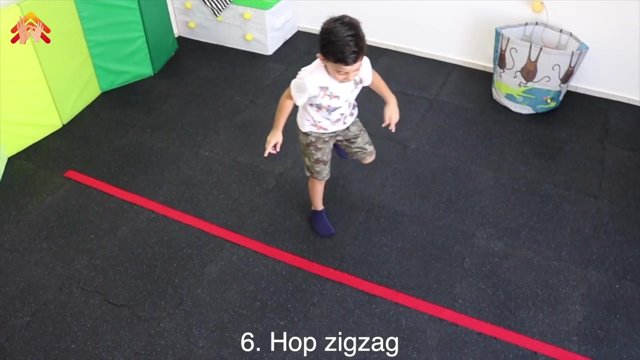 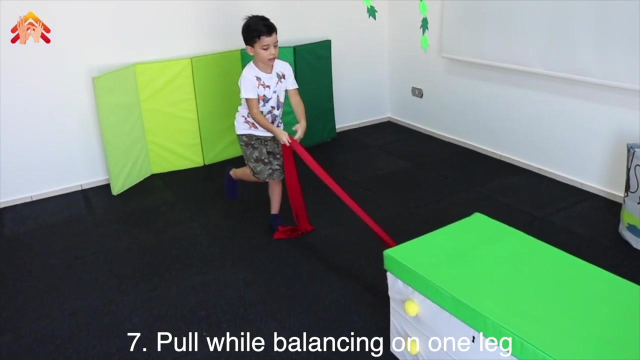 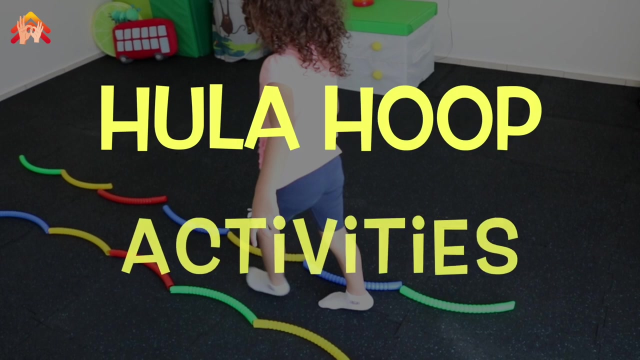 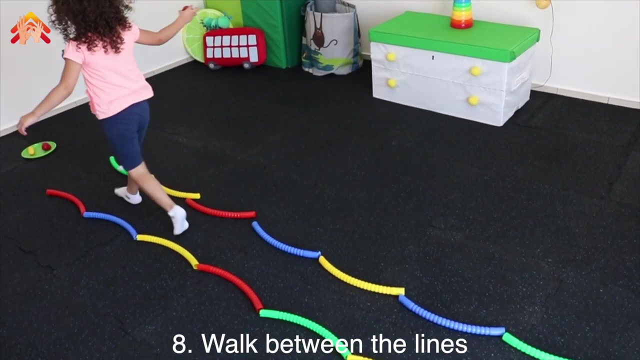 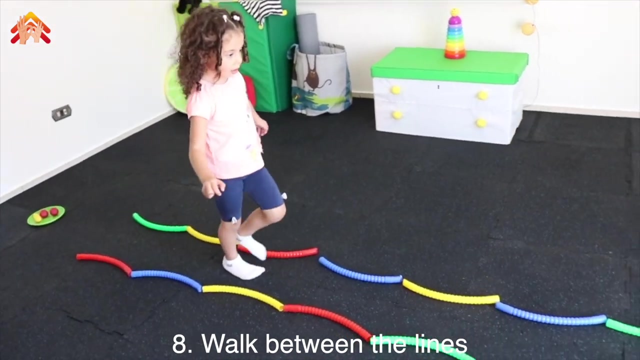 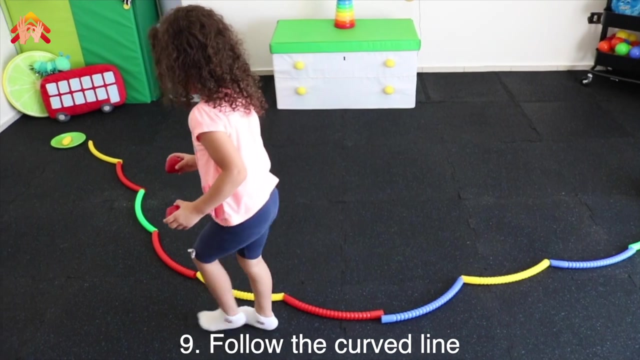 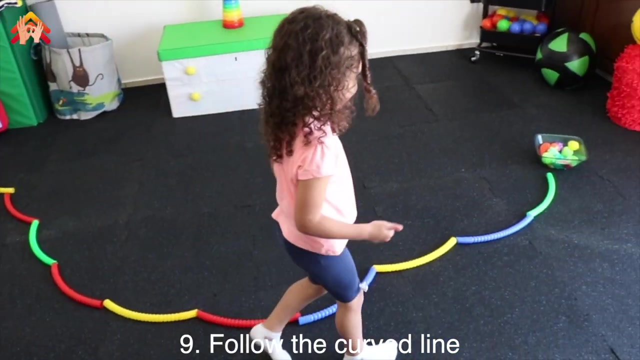 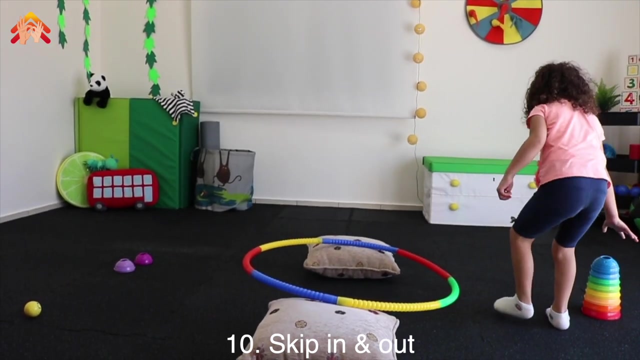 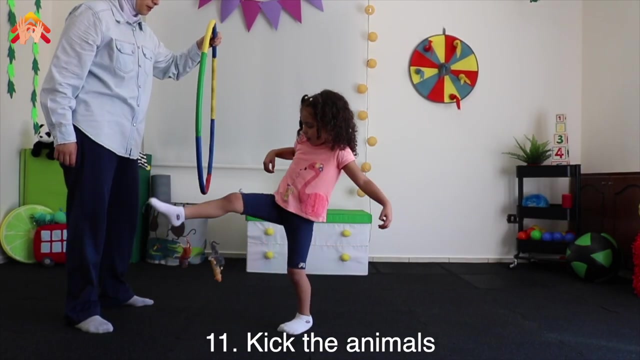 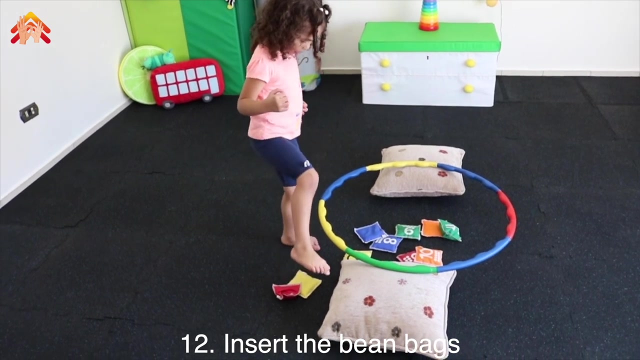 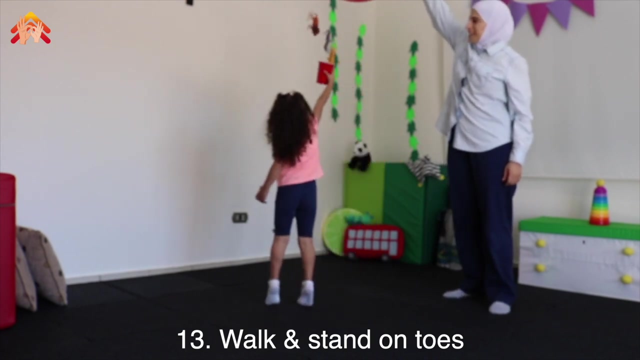 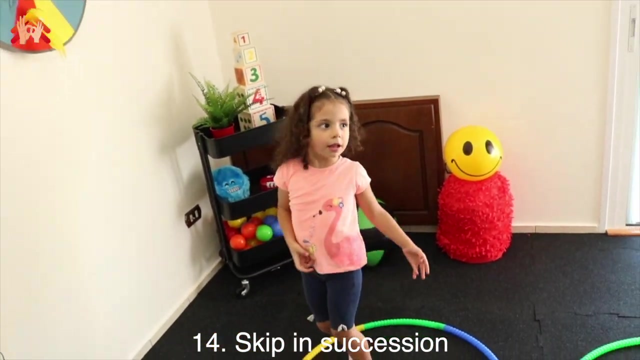 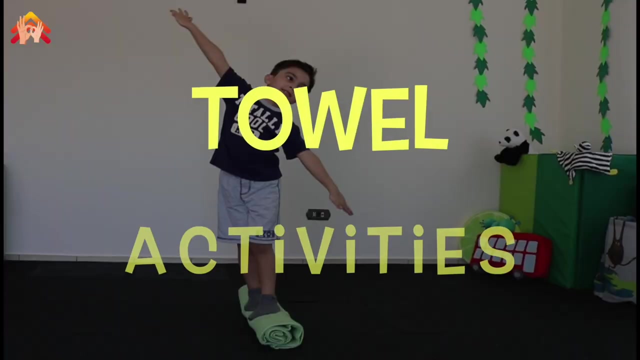 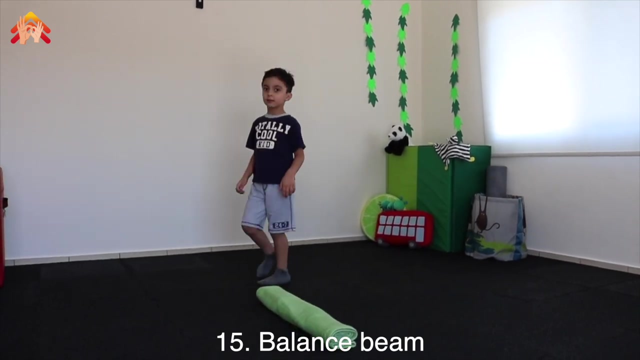 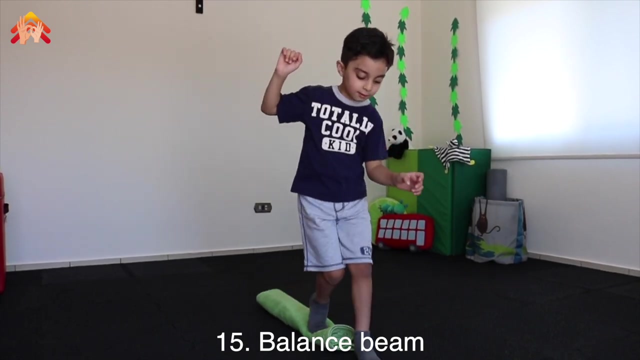 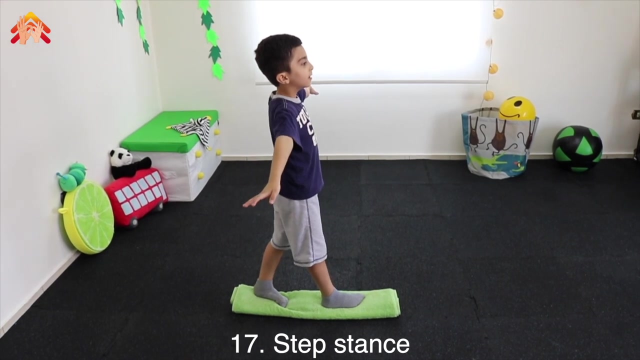 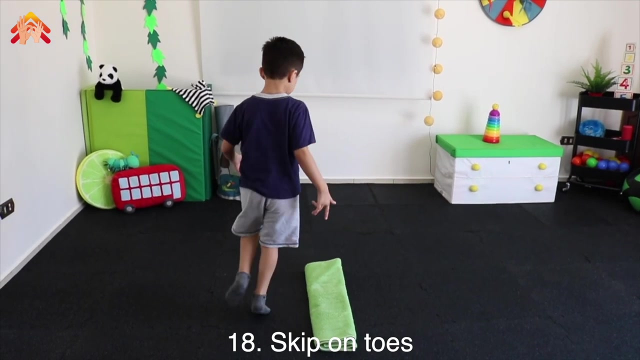 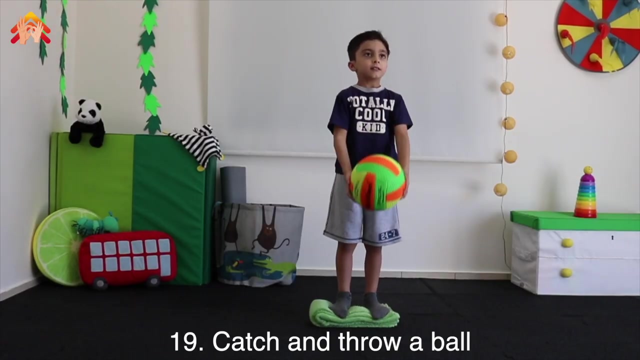 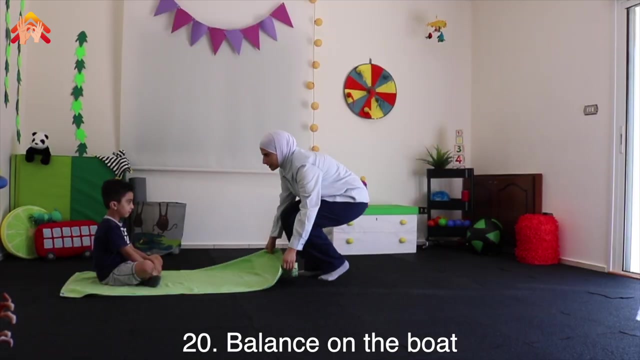 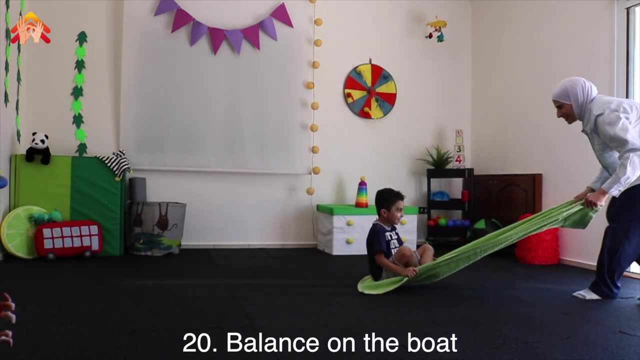 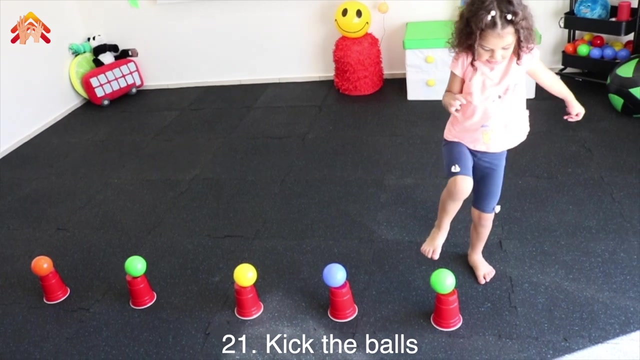 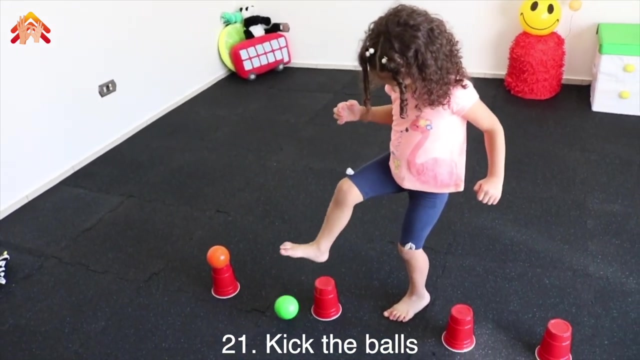 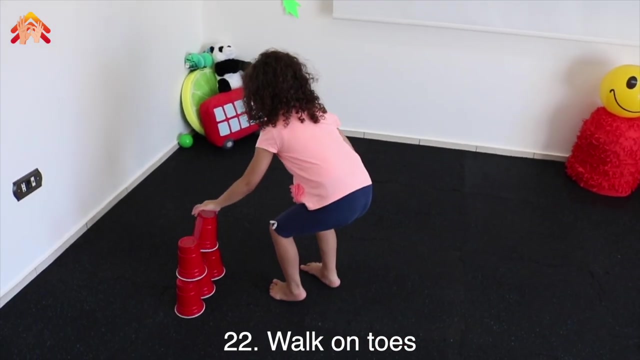 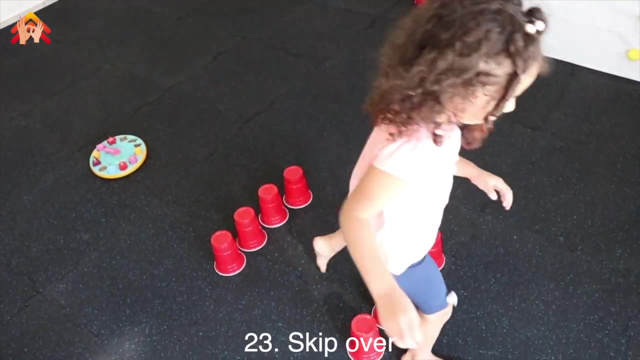 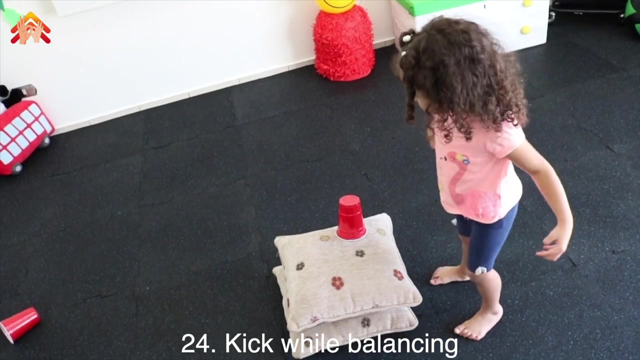 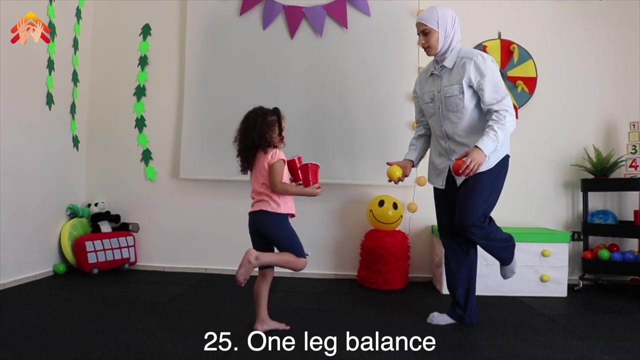 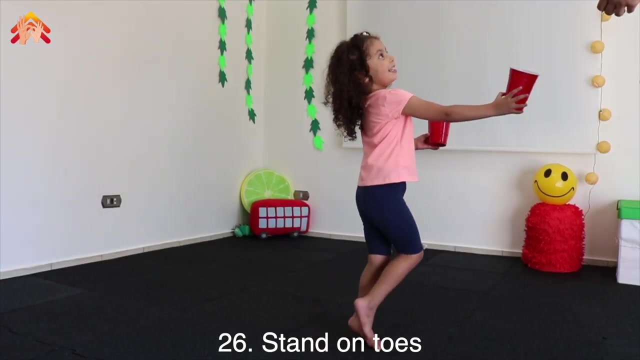 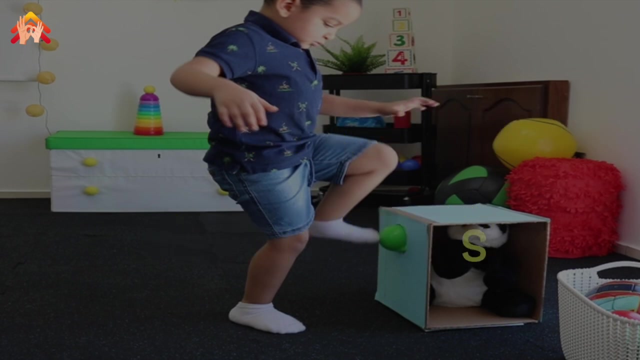 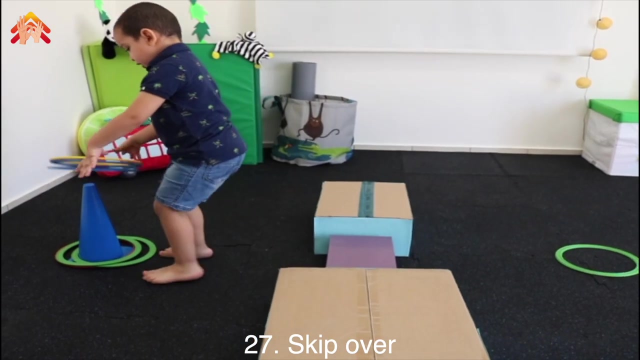 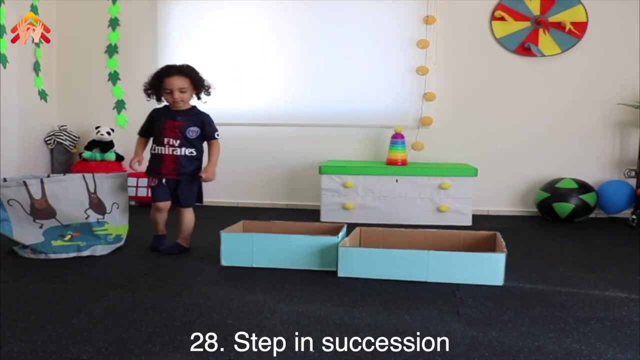 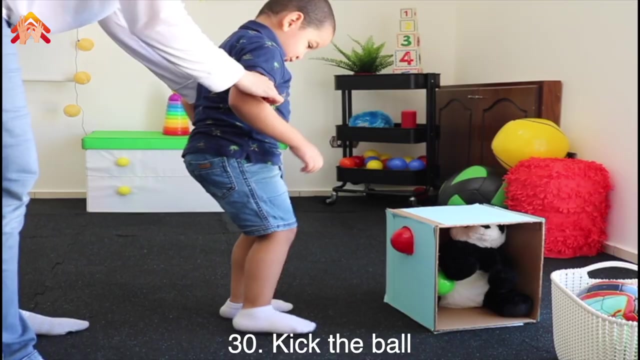 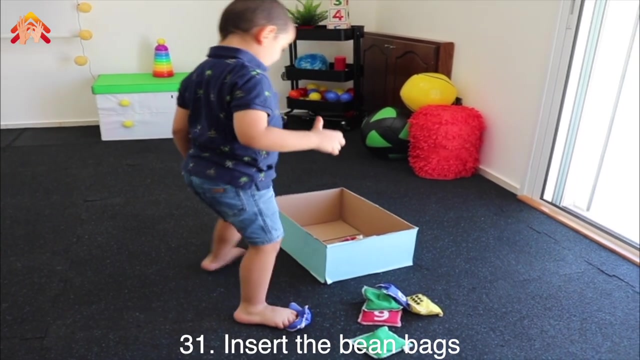 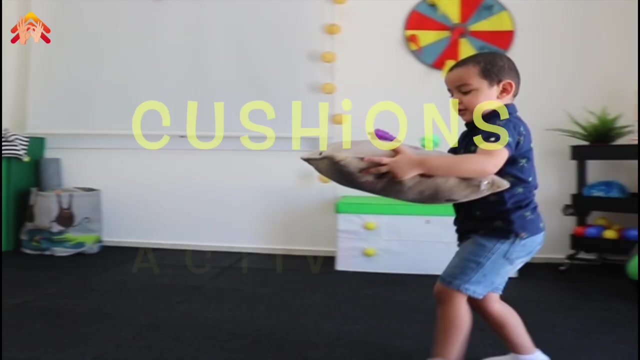 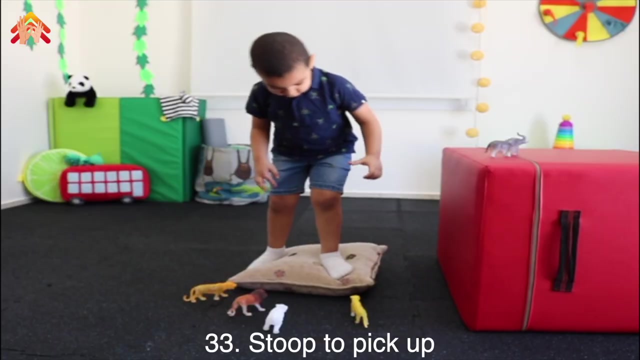 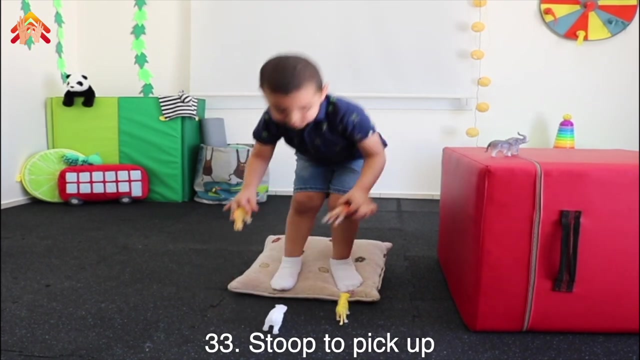 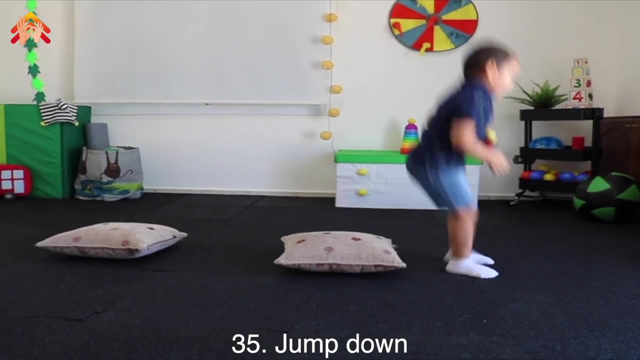 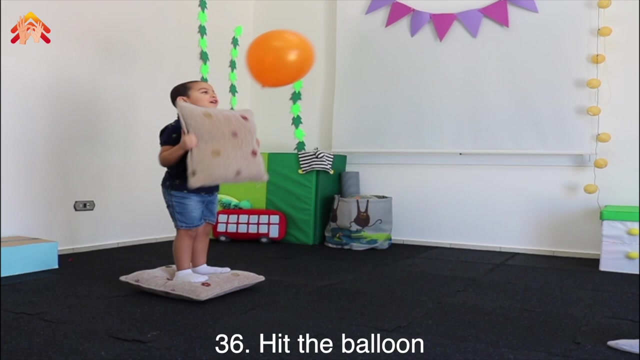 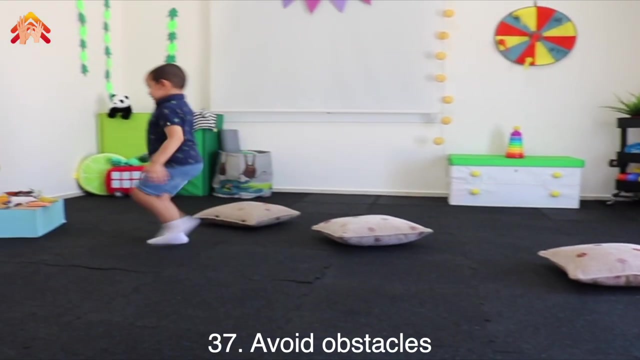 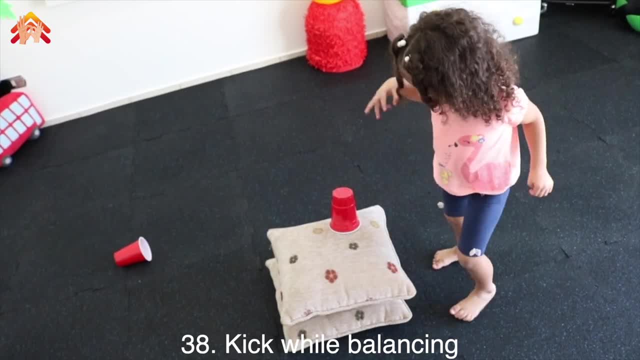 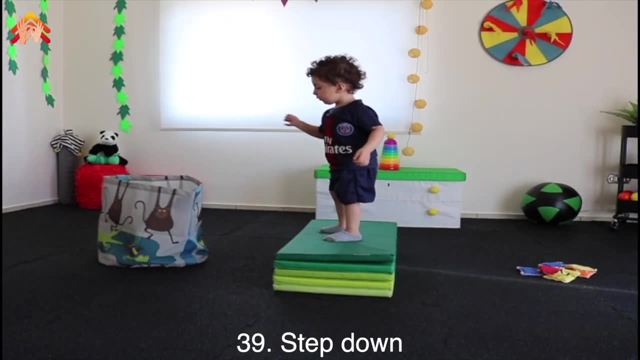 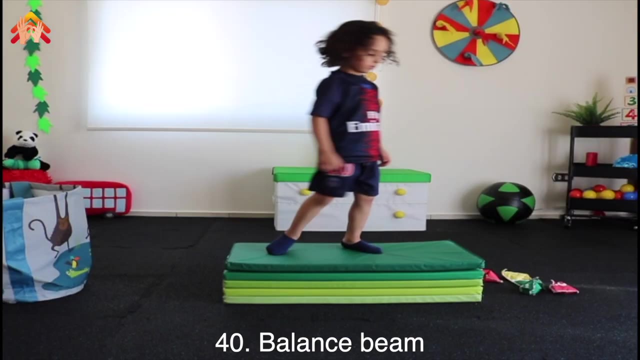 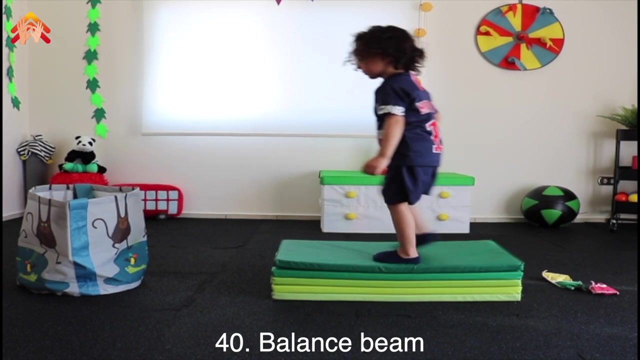 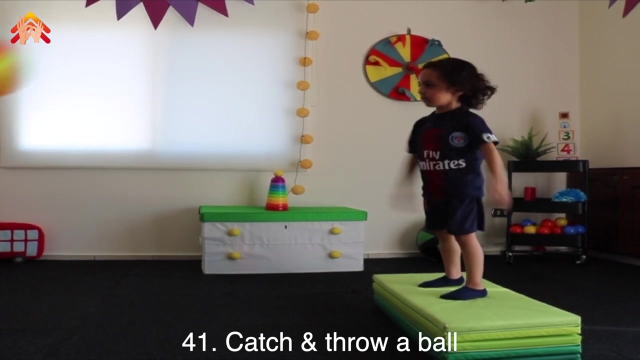 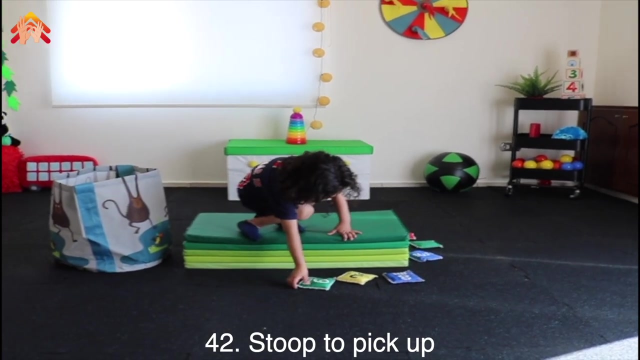 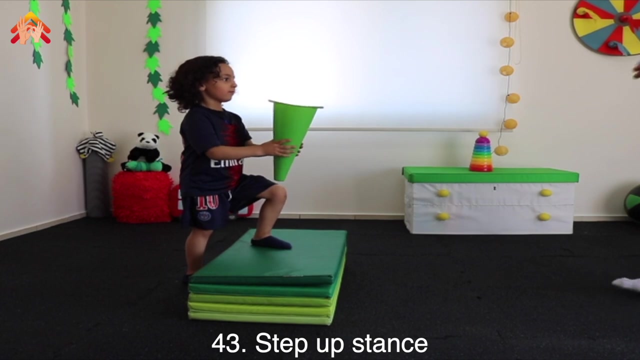 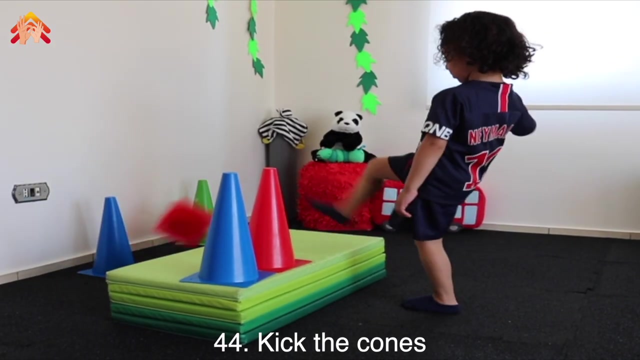 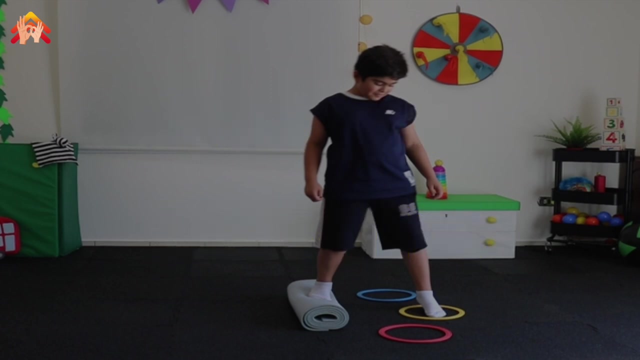 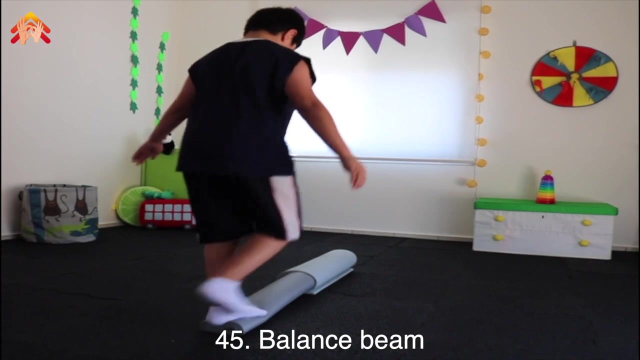 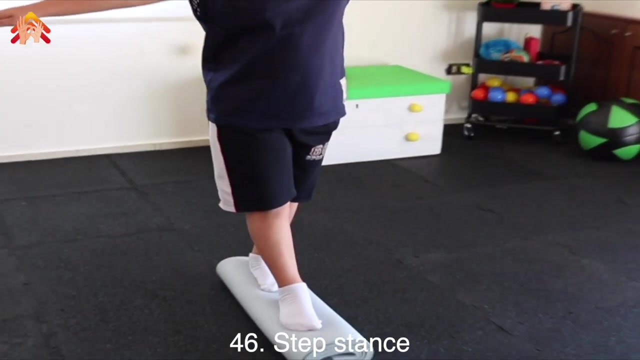 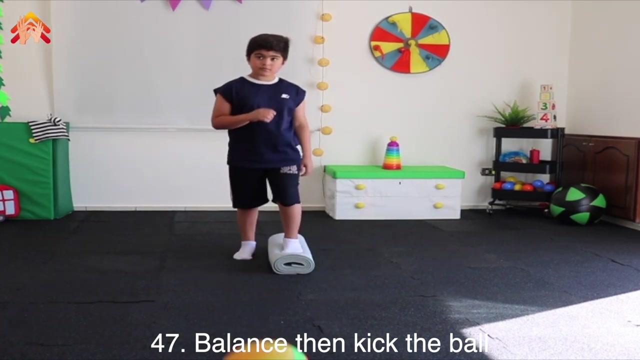 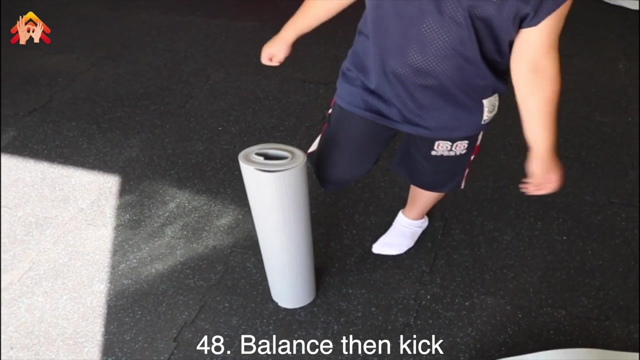 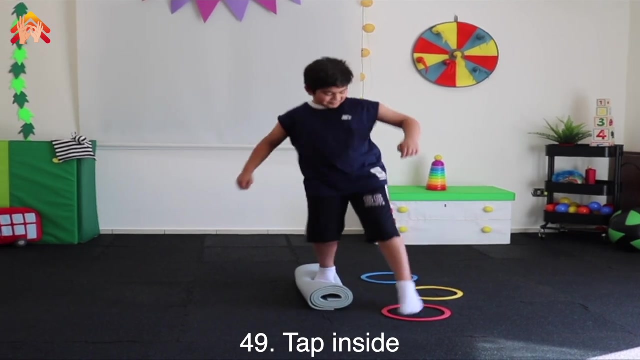 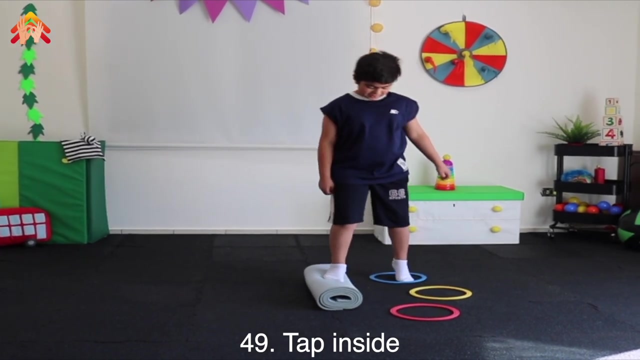 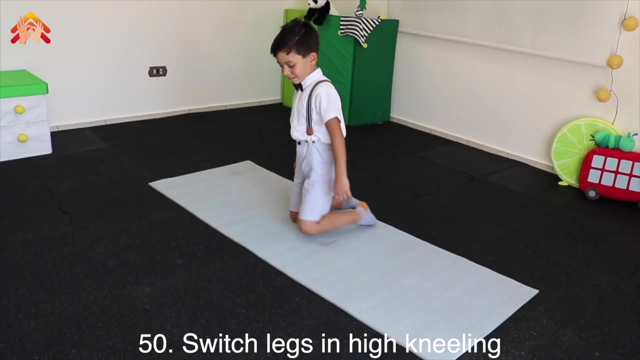 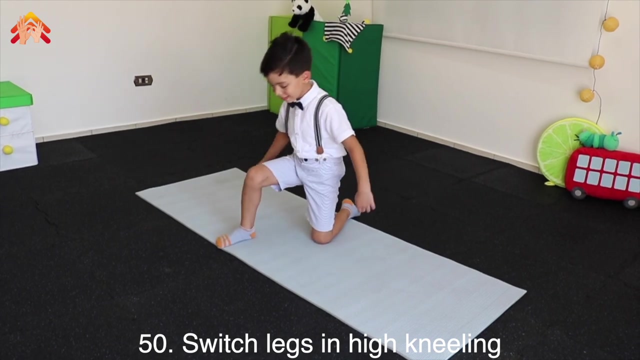 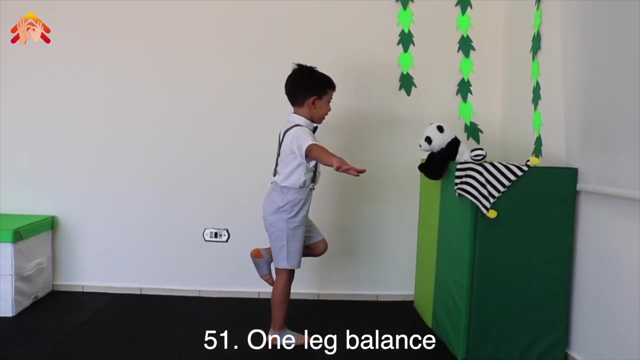 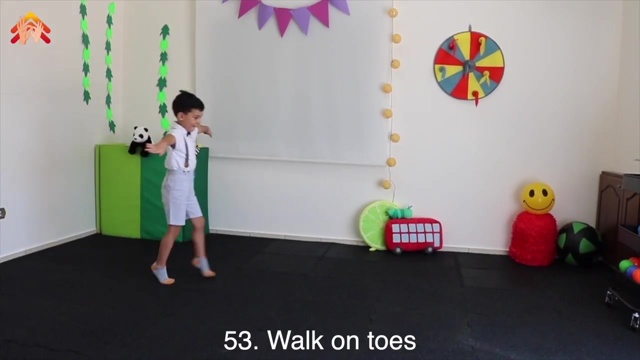 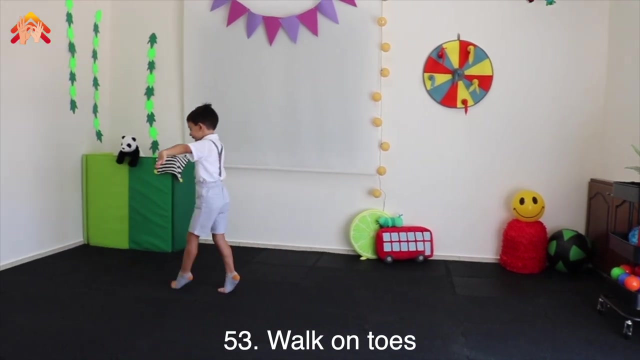 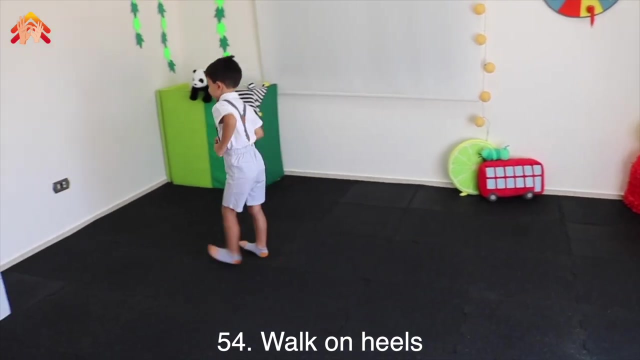 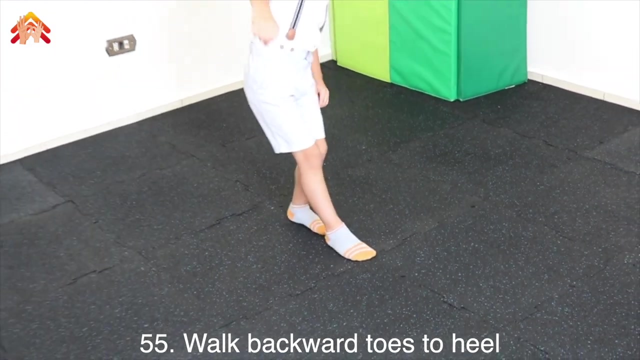 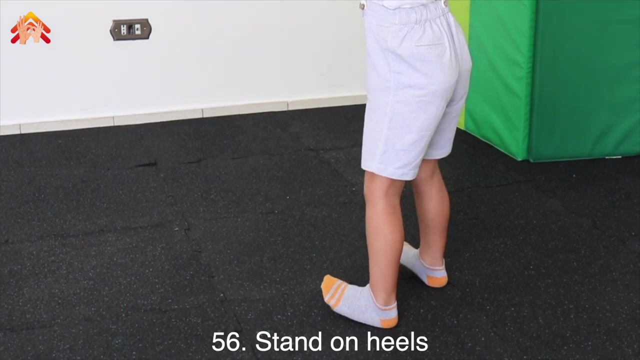 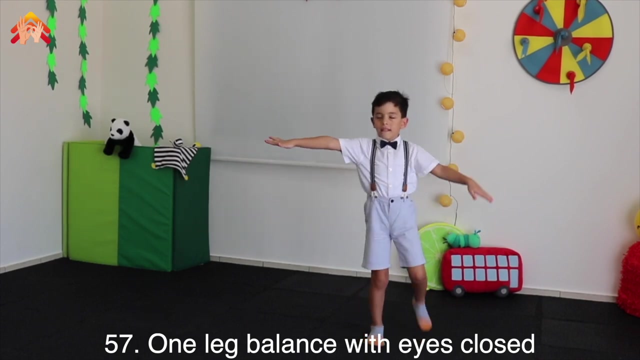 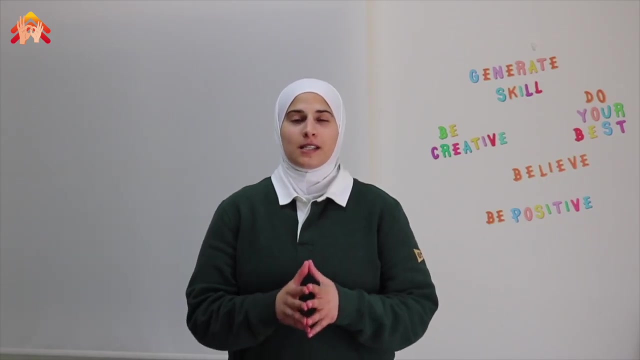